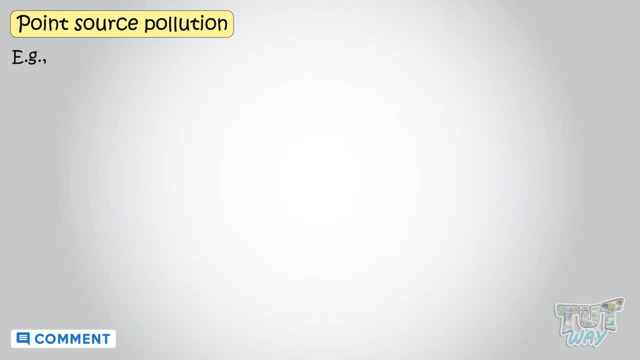 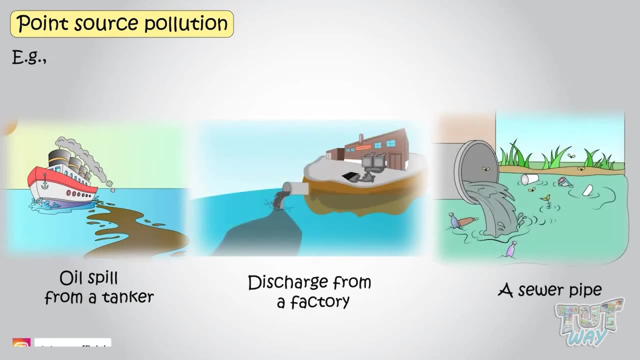 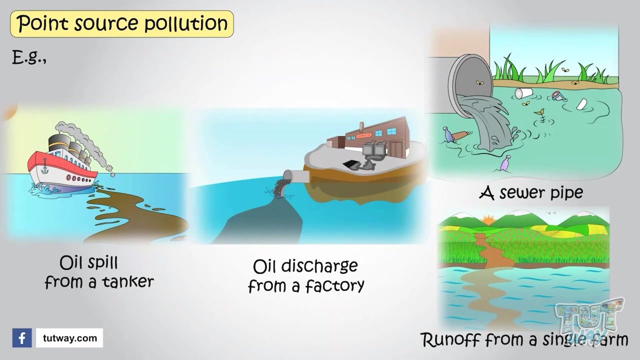 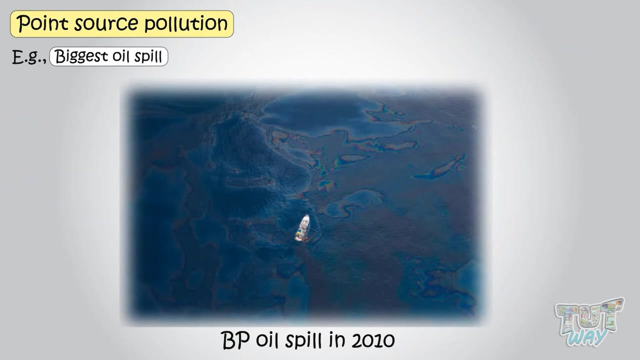 Other examples of point source pollution include an oil spill from a tanker, Discharge from a factory, A sewer pipe Runoff from a single farm. So these are point source pollution occurring from a single location. BP oil spill in 2010 is an example of point source pollution. 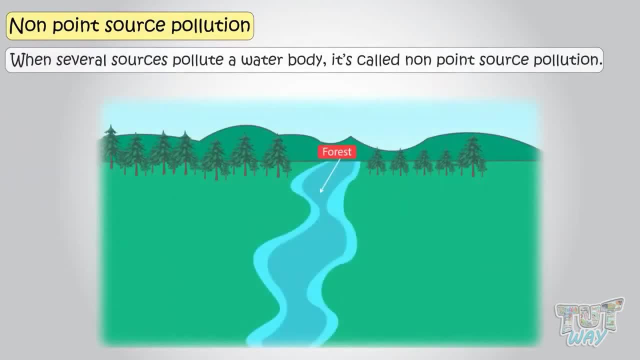 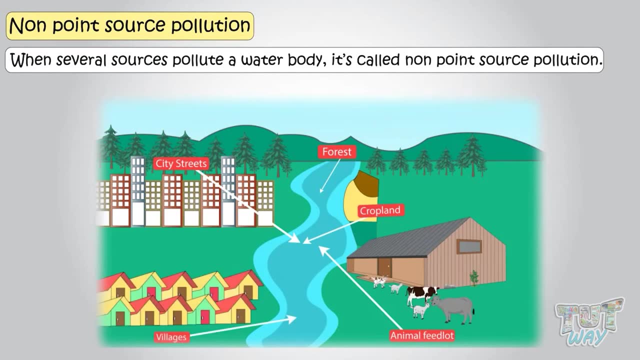 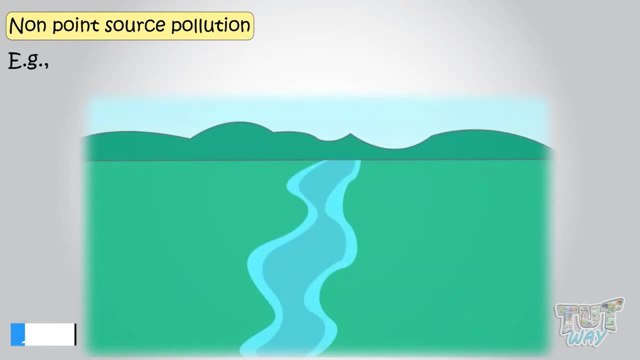 When not one but several sources of pollution are there that are contributing in polluting a water body. Let's look at the examples body. It's called non-point sources of pollution. For example, one body may be contaminated by multiple sources, like agricultural runoff, city street runoff, construction sites and. 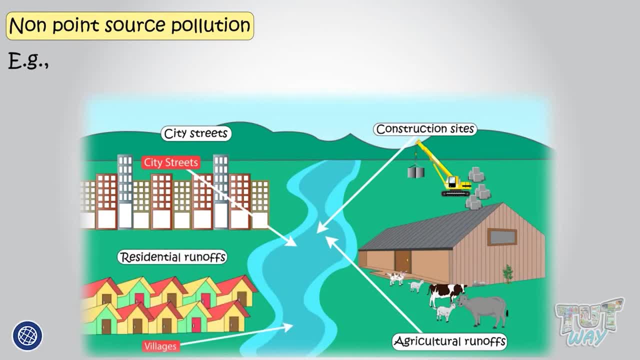 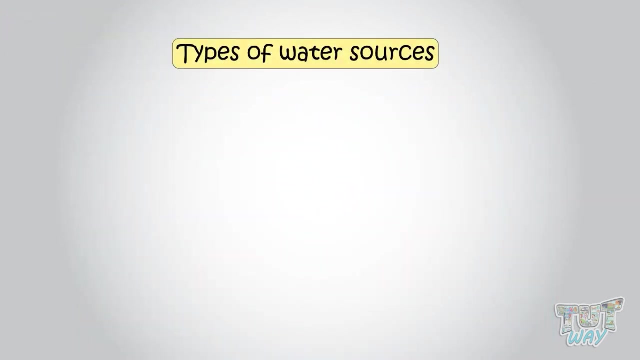 residential runoffs. The Mississippi River is at great risk for non-point source pollution because it is so large and it is exposed to a variety of pollution sources. We learned types of water pollution. now Let's learn types of water sources. Water sources can be divided into surface waters and groundwaters, All 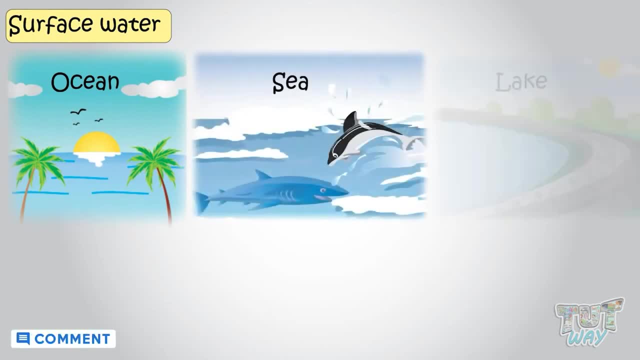 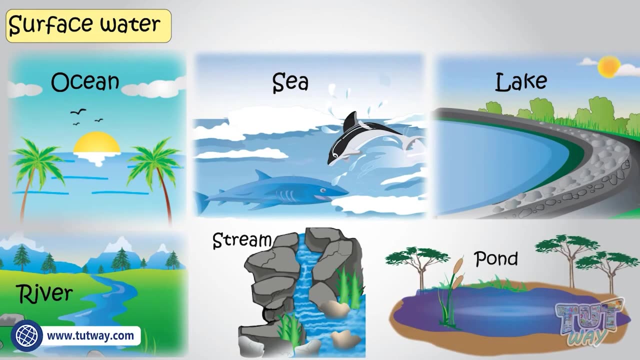 the water bodies like ocean, seas, lakes, rivers, etc. can be divided into surface waters and groundwaters. All the water bodies like ocean, seas, lakes, rivers, streams and ponds are surface waters, that is, they exist on the surface of Earth. 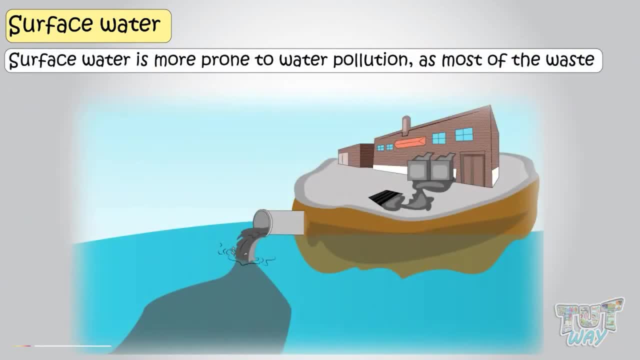 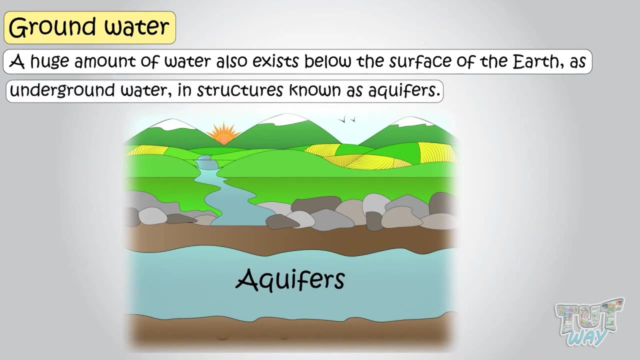 Surface waters are more prone to water pollution, as most of the waste discharge is left into the surface waters. A huge amount of water also exists below the surface of the earth as underground water, In the underground rock structures known as aquifers, which we cannot see, and seldom think about water stored. 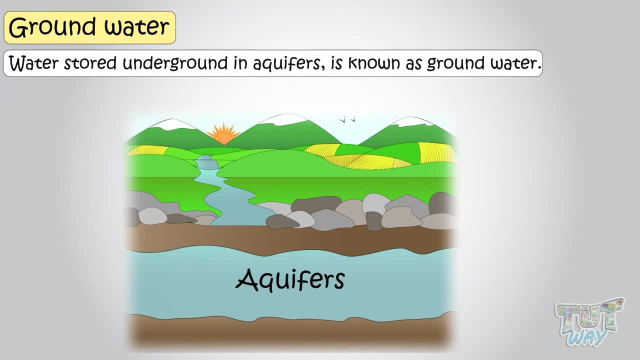 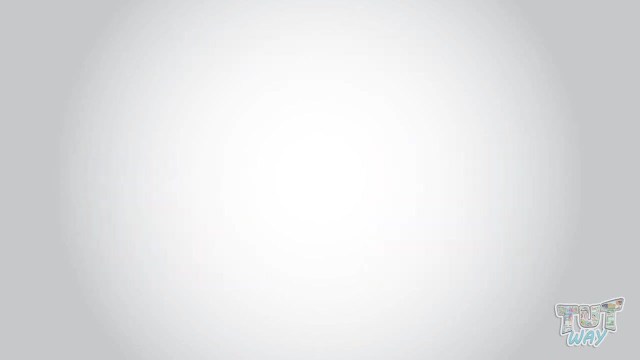 underground in aquifers, is known as groundwater. groundwater is less prone to water pollution, but it is also getting polluted. so, kids, today we learn what is water pollution, what are the types of water sources and also types of water pollution. now you may go ahead and take a quiz to learn more. bye, bye, thank you.